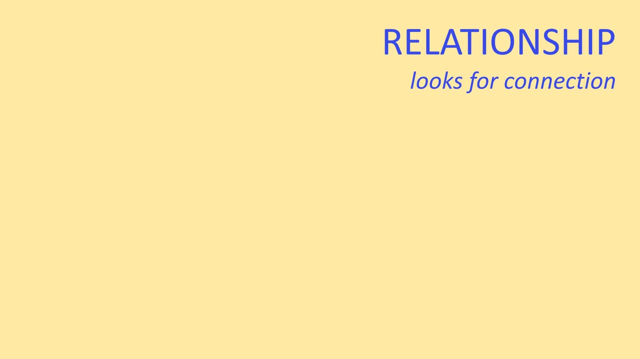 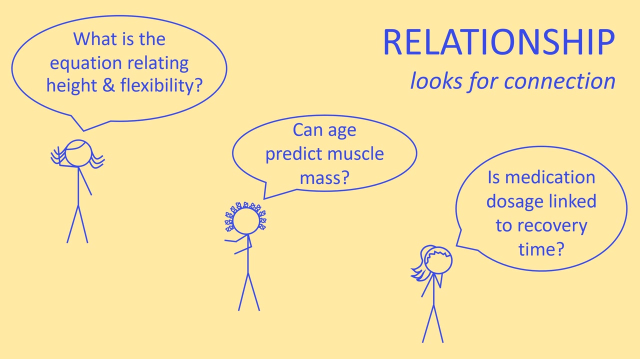 Relationship, on the other hand, could look like, for example, looking for an equation between height and flexibility, Or asking whether age predicts muscle mass. We're trying to see if medication dosage is linked to recovery time. In every one of these scenarios, we're seeking out correlation or causation, or some sort of prediction. 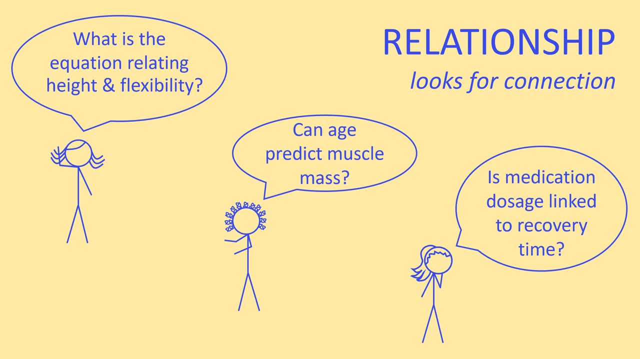 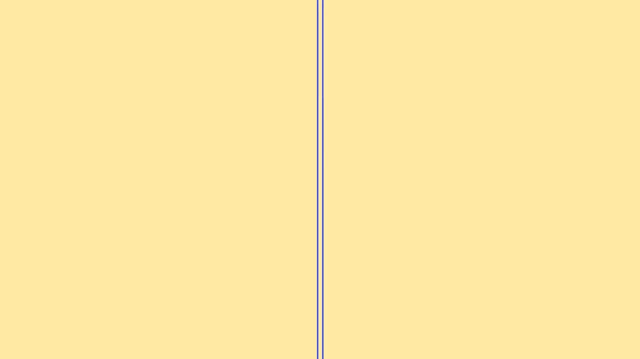 from one group to another. The second thing we have to evaluate after purpose is the type of data we're looking at, And the two main categories are categorical and continuous. Categorical data is qualitative. Even if there are numbers attached, those values don't represent any numerical meaning. 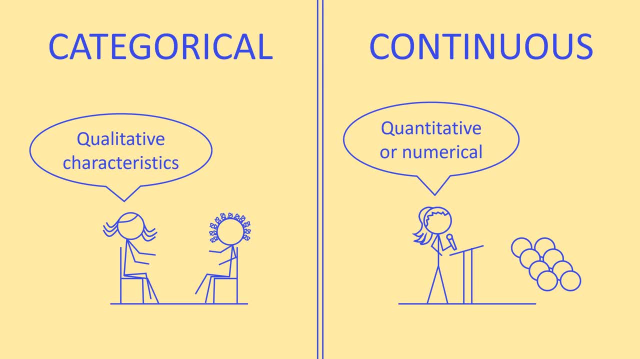 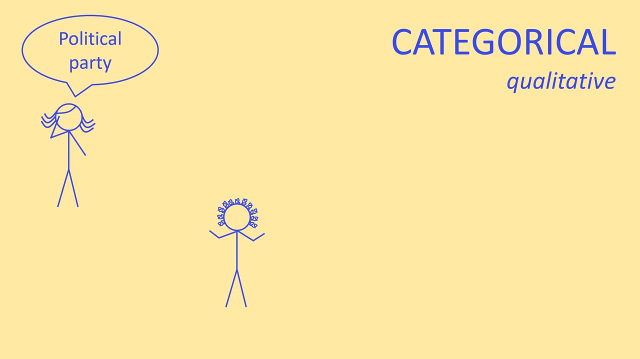 Continuous data, on the other hand, is quantitative or numerical. As you increase the value, that represents an increasing amount of that property. Categorical qualities could look like political party, or even a yes or no answer, Or it could be which gene was expressed. 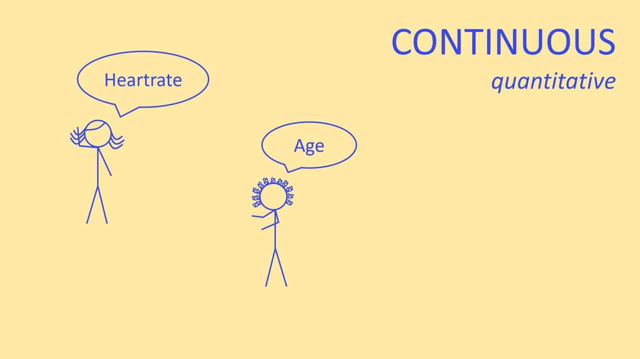 On the other hand, if your data involves things like heart rate, age or number of bacterial colonies, then you're looking at continuous data. Even in that last example, the number of colonies would only be an integer value, But that still qualifies as continuous data in statistics. 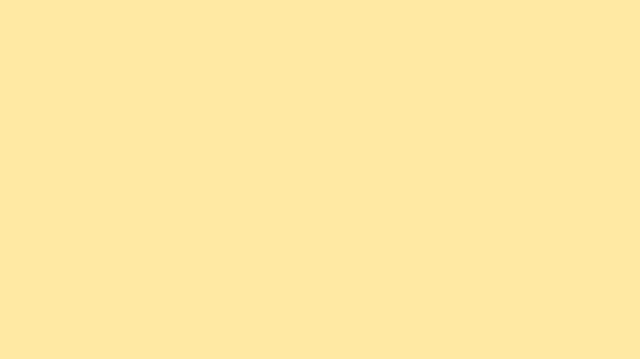 Once you figure out your experiment's purpose and type of data, you can choose between three main families of statistical tests. Those families include the chi-squared family, the t-test or ANOVA family and the correlation family. Remember, purpose has two choices. 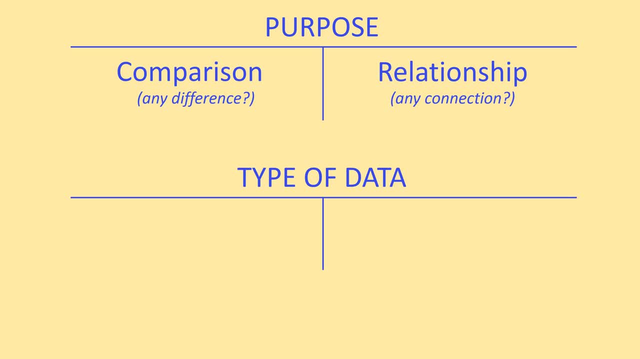 Comparison relationship. Type of data could be either categorical or continuous. If your experiment is trying to draw a comparison or find a difference and you only have categorical data, then you can almost guarantee that you will be working in the chi-squared family. 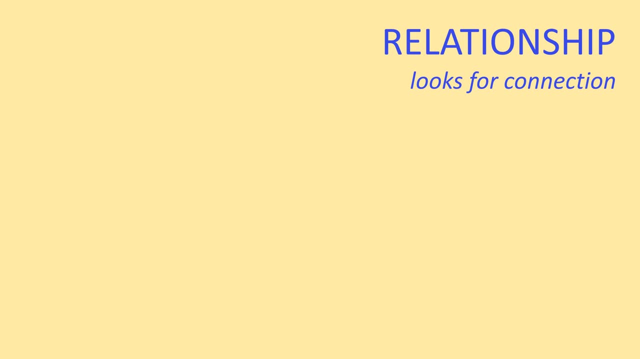 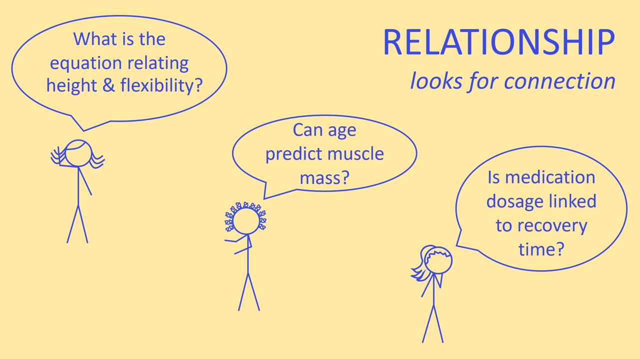 Relationship, on the other hand, could look like, for example, looking for an equation between height and flexibility, or asking whether age predicts muscle mass. We're trying to see if medication dosage is linked to recovery time. In every one of these scenarios, we're seeking out correlation or causation. 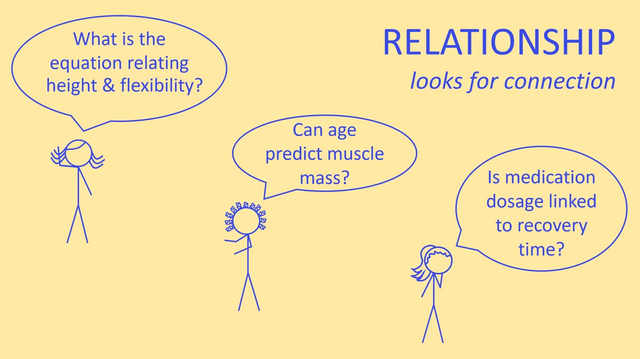 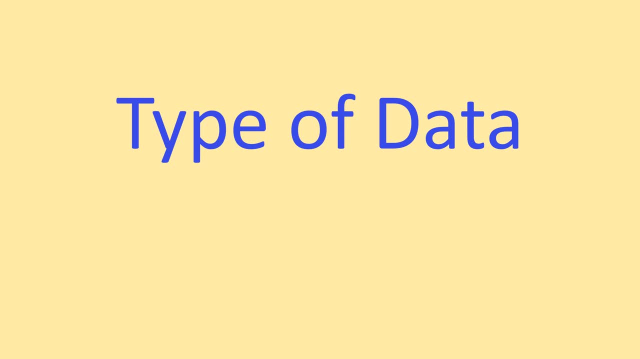 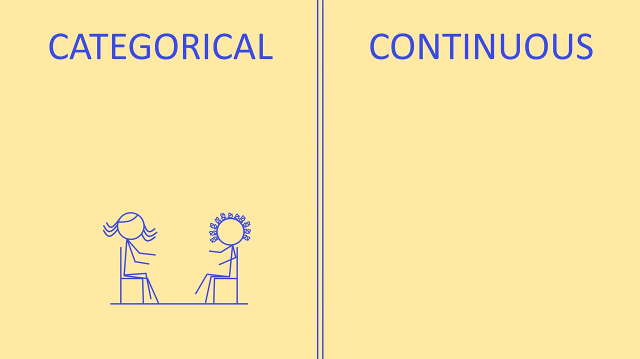 or some sort of prediction from one group to another. The second thing we have to evaluate after purpose is the type of data we're looking at, And the two main categories are categorical and continuous. Categorical data is qualitative. Even if there are numbers attached, those values don't represent any numerical meaning. 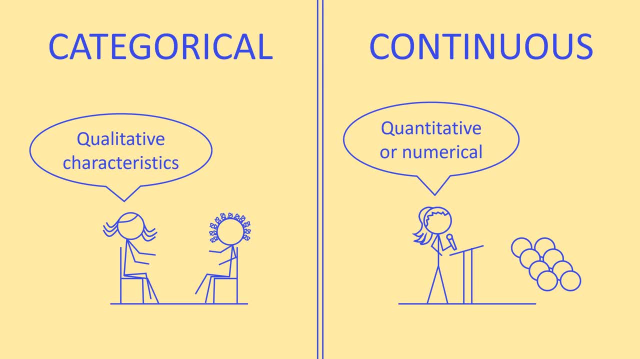 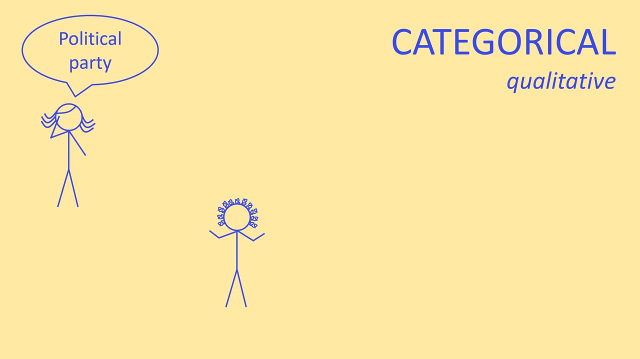 Continuous data, on the other hand, is quantitative or numerical. As you increase the value, that represents an increasing amount of that property. Categorical qualities could look like political party, or even a yes or no answer, Or it could be which gene was expressed. 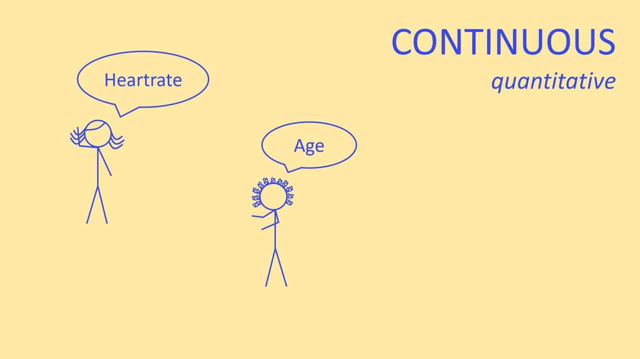 On the other hand, if your data involves things like heart rate, age or number of bacterial colonies, you're looking at continuous data. Even in that last example, the number of colonies would only be an integer value, but that still qualifies as continuous data in statistics. 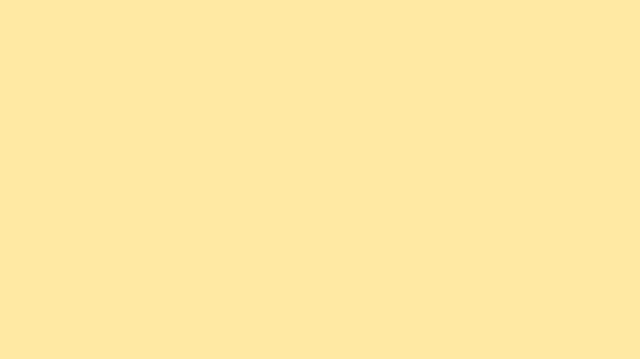 Once you figure out your experiment's purpose and type of data, you can choose between three main families of statistical tests. Those families include the chi-squared family, the t-test or ANOVA family and the correlation family. Remember, purpose has two choices. 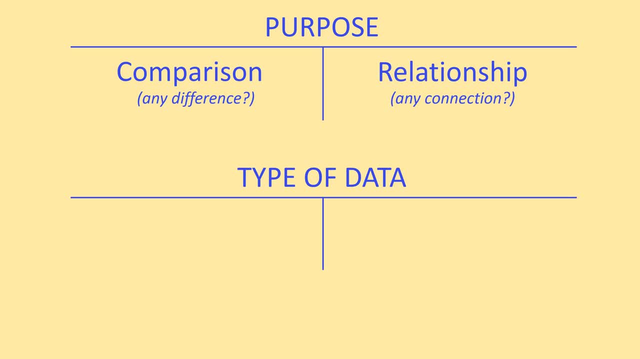 Comparison relationship. Type of data could be either categorical or continuous. If your experiment is trying to draw a comparison or find a difference and you only have categorical data, then you can almost guarantee that you will be working in the chi-squared family. 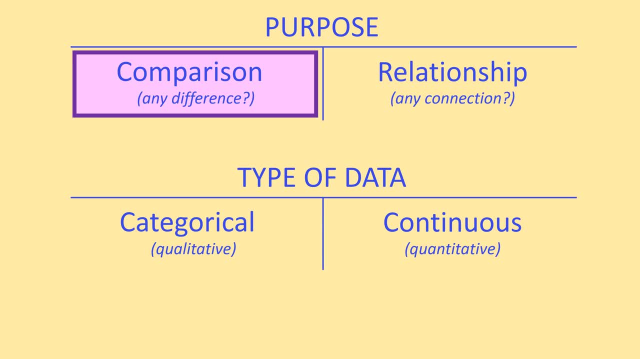 On the other hand, if you're drawing a comparison or finding a difference, but your data has categorical and continuous types, that would be the t-test family. What does it mean to be categorical and continuous? Well, maybe you are trying to compare the mean height. 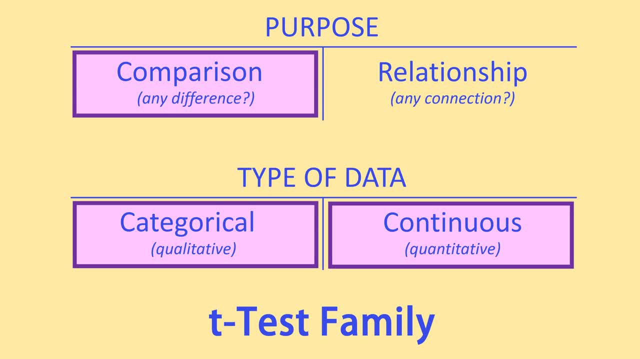 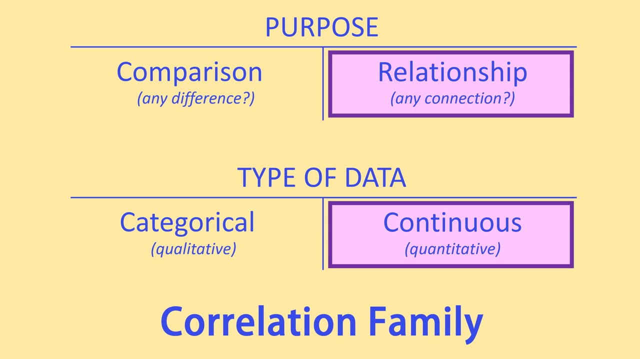 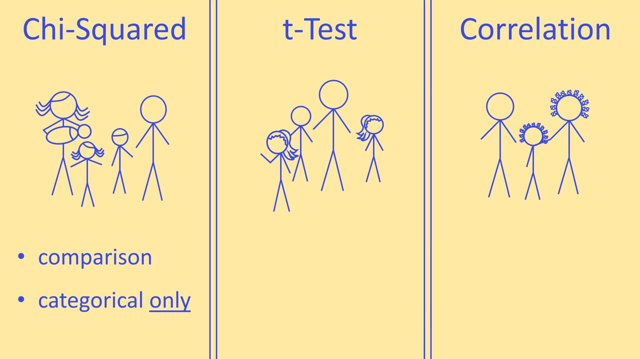 of different groups of people. The groups qualify as categorical height. that's continuous. On the other hand, if you're trying to find a relationship between continuous variables, then you are definitely in the correlation family. Here are our three families and, to summarize, 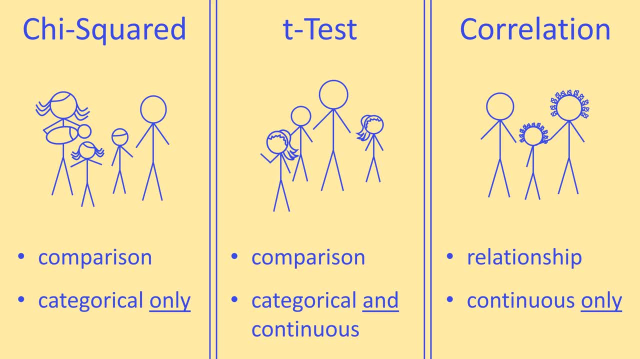 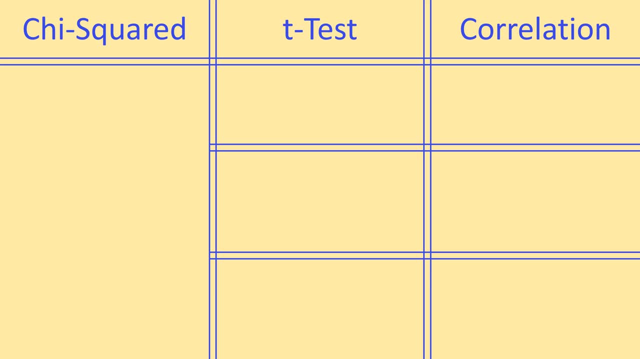 here are the typical characteristics. Once you know which family you're dealing with, you can start to drill down to find a particular test that's appropriate for your experiment. Chi-squared is easy because there are the same two tests for any number of groups or levels. 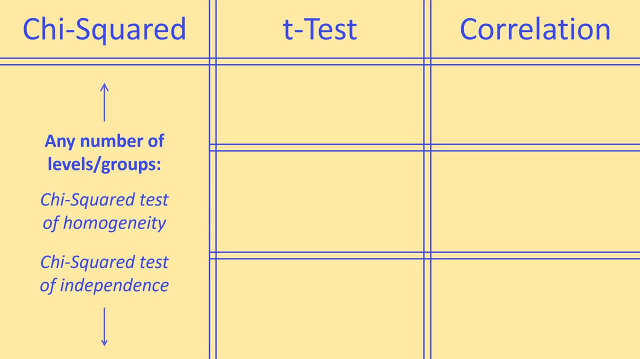 In the t-test family. we have to know how many groups does our independent variable consider? If you're only looking at one sample group, you would use a one-sample t-test. That would be the case for an experiment where you're trying to compare the mean height at your high school. 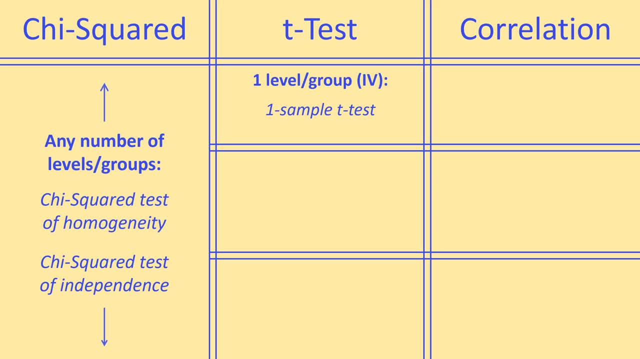 to the US population for teenagers. In this case you have a known average. you know the population average for all teenagers in the US and you're comparing it to one sample from your high school. On the other hand, maybe your experiment involves two groups or two levels. 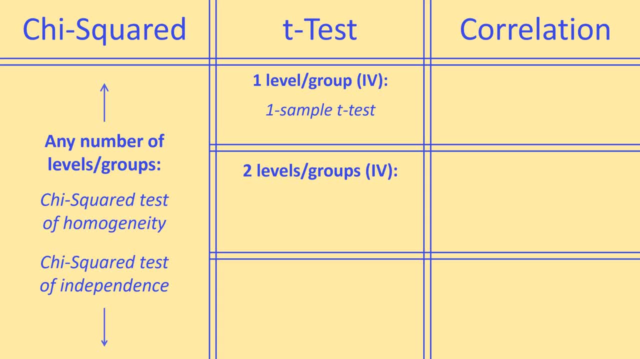 of the independent variable. For example, perhaps you're comparing the mean height of men to women and you're trying to figure out whether there's a difference. In that case you would use a two-sample unpaired t-test. There is another kind. 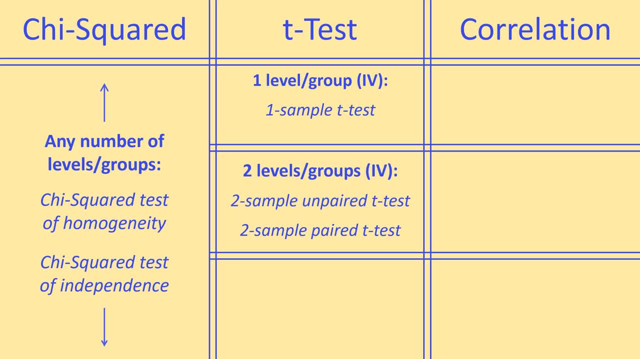 a two-sample paired t-test And that's for scenarios where you test the same group twice. For example, maybe you have a group of people and you give them a memory task before doing an exercise and then you give them another memory task after doing an exercise. 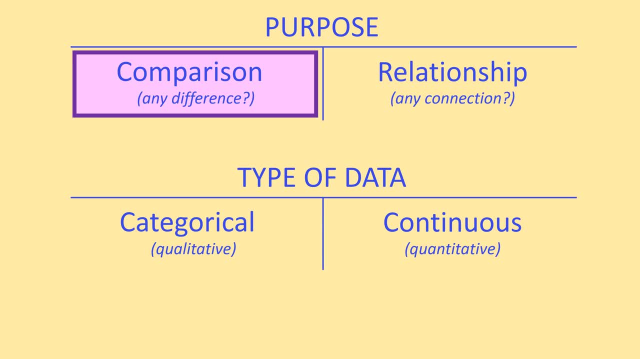 On the other hand, if you're drawing a comparison or finding a difference, but your data has categorical and continuous types, that would be the t-test family. What does it mean to be categorical and continuous? Well, maybe you are trying to compare the mean height. 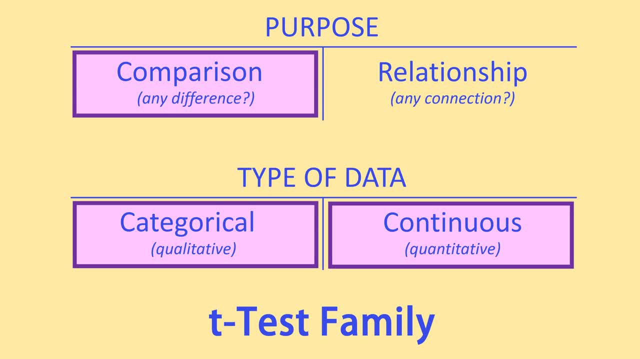 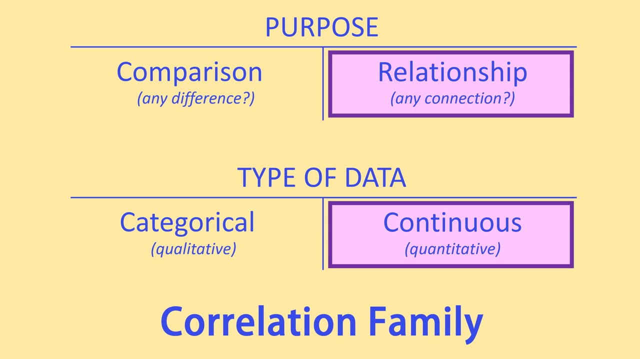 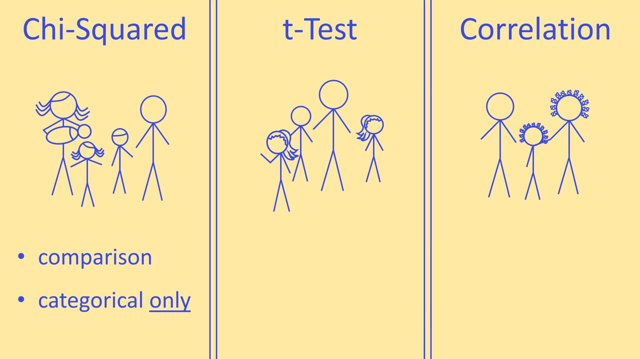 of different groups of people. The groups qualify as categorical Height, that's continuous. On the other hand, if you're trying to find a relationship between continuous variables, then you are definitely in the correlation family. Here are our three families and, to summarize, 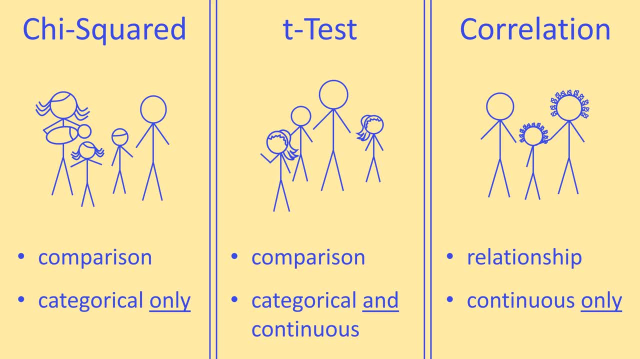 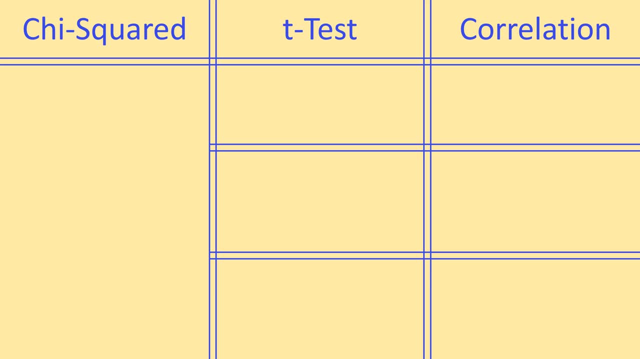 here are the typical characteristics. Once you know which family you're dealing with, you can start to drill down to find a particular test that's appropriate for your experiment. Chi-squared is easy because there are the same two tests for any number of groups or levels. 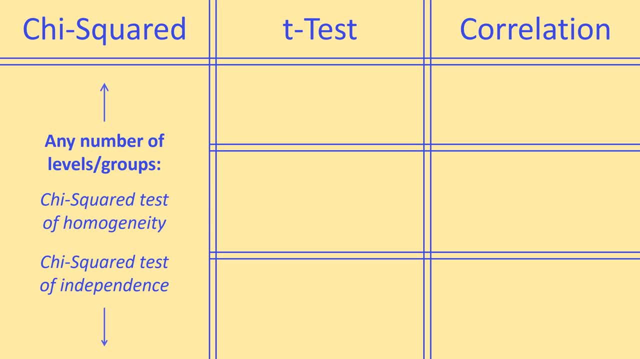 In the t-test family. we have to know how many groups does our independent variable consider? If you're only looking at one sample group, you would use a one-sample t-test. That would be the case for an experiment where you're trying to compare the mean height at your high school. 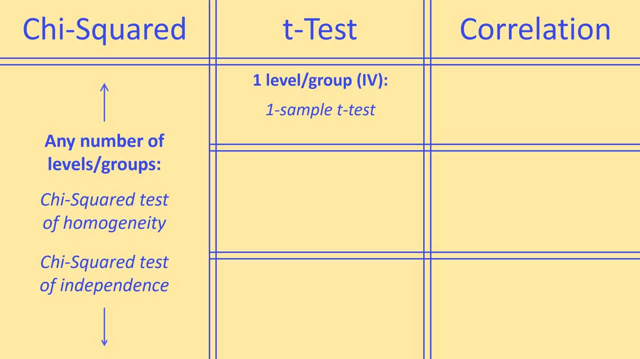 to the US population for teenagers. In this case you have a known average. You know the population average for all teenagers in the US and you're comparing it to one sample from your high school. On the other hand, maybe your experiment involves two groups. 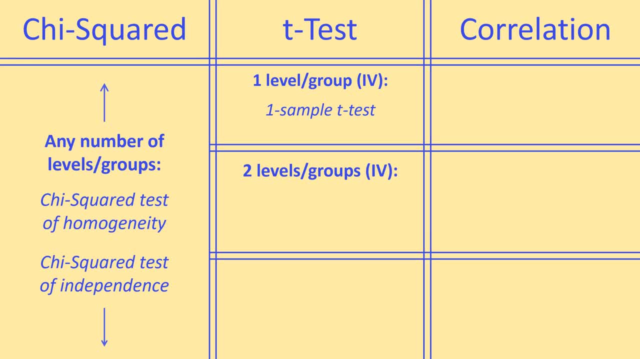 or two levels of the independent variable. For example, perhaps you're comparing the mean height of men to women and you're trying to figure out whether there's a difference. In that case, you would use a two-sample unpaired t-test. 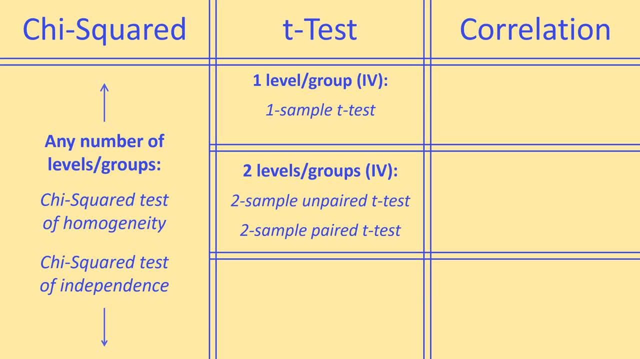 There is another kind, a two-sample paired t-test, and that's for scenarios where you test the same group twice. For example, maybe you have a group of people and you give them a memory task before doing an exercise and then you give them another memory task after doing an exercise. 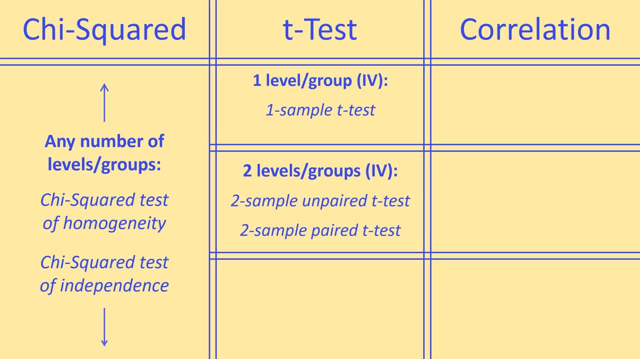 And you're trying to find out. did the exercise make a difference? You're looking for a difference. In that case, your data points have specific pairing and you're looking for a difference. You're looking for an improvement. So this is the scenario where you would use a paired t-test. 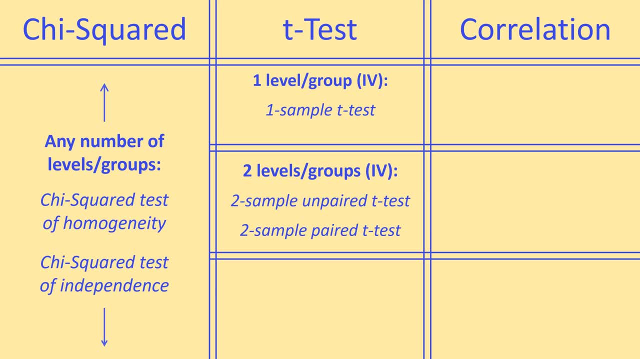 But it doesn't have to be the same group. For example, your pairing might involve mothers and daughters, or it could be any two groups the experimenter specifically paired together. If you have more than two groups, so three or more, you'll be using a one-way ANOVA test. 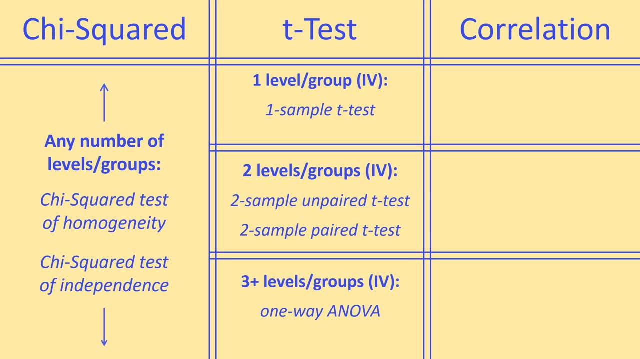 this stands for analysis of variance. This test looks to see whether or not they are all similar. If you have any one group that is different, you'll get a statistically significant result from this test. But the thing about one-way ANOVA tests: 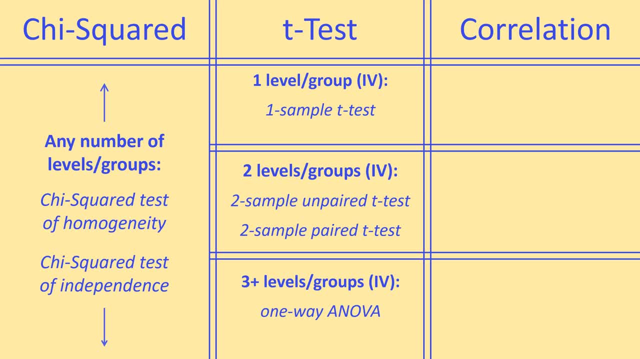 is. it doesn't tell you which of the three groups, or which of the four groups, or five or however many. it doesn't tell you which one is statistically different or if there are multiple that are statistically different from each other. This test only looks for. 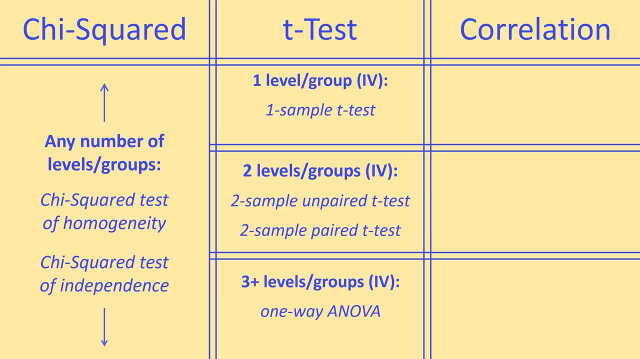 whether or not they're all similar or at least one is different, On to the final family. We will consider just the scenario where you have one independent variable and one dependent variable. In those circumstances, there are two primary tests you might look for. 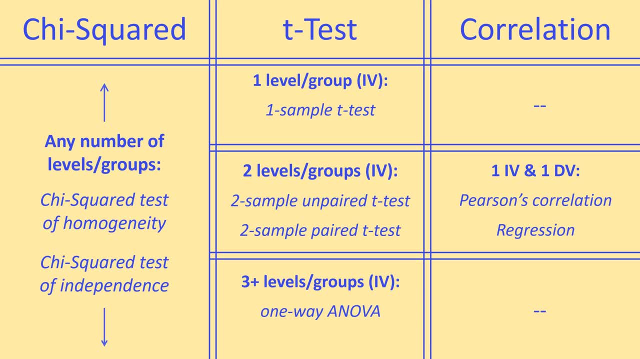 Pearson's correlation and regression Correlation tries to figure out how closely connected the two variables are. Is height a predictor of flexibility? Does age correlate with muscle mass? So it tries to understand how well those variables go together, If you know one. 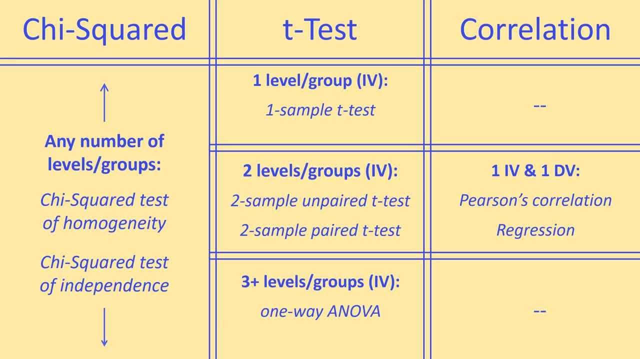 can you predict the other one really, really well? Do they correlate strongly or do they correlate poorly? That's what correlation tries to understand. On the other hand, regression tries to figure out a specific mathematical equation that describes the relationship. So it doesn't just want to know. 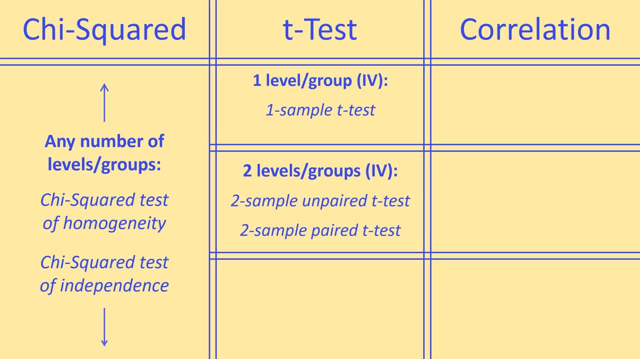 And you're trying to find out. did the exercise make a difference? You're looking for a difference. In that case, your data points have specific pairing and you're looking for a difference. You're looking for an improvement. So this is the scenario where you would use a paired t-test. 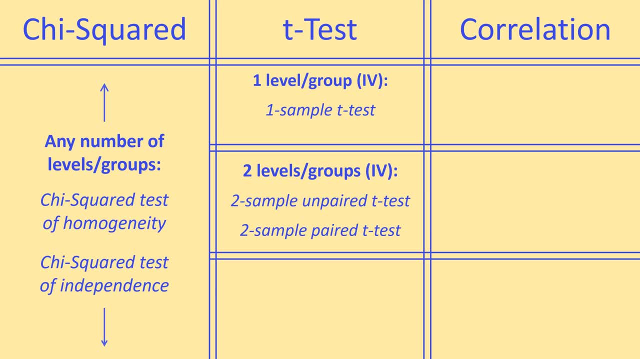 But it doesn't have to be the same group. For example, your pairing might involve mothers and daughters, or it could be any two groups the experimenter specifically paired together. If you have more than two groups, so three or more, you'll be using a one-way ANOVA test. 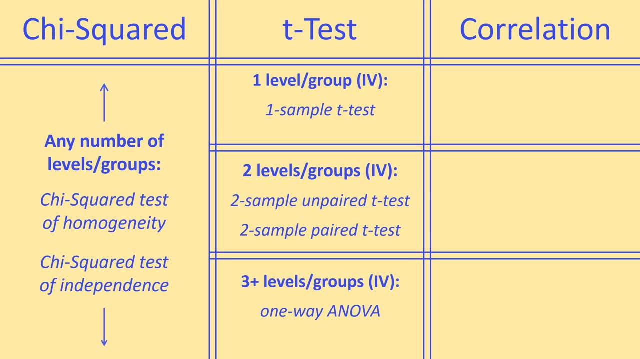 This stands for analysis of variance. This test looks to see whether or not they are all similar. If you have any one group that is different, you'll get a statistically significant result from this test. But the thing about one-way ANOVA tests: 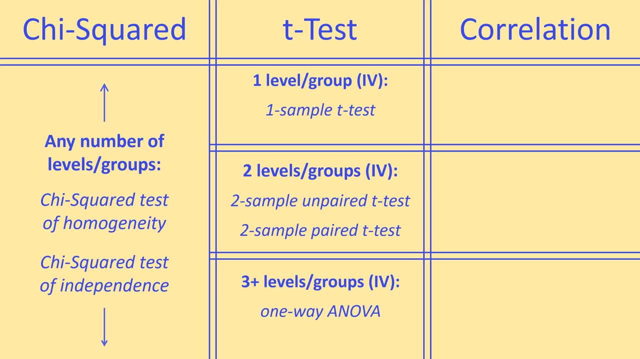 is. it doesn't tell you which of the three groups or which of the four groups or five or however many. it doesn't tell you which one of the three groups or one is statistically different, or if there are multiple that are statistically different from each other. 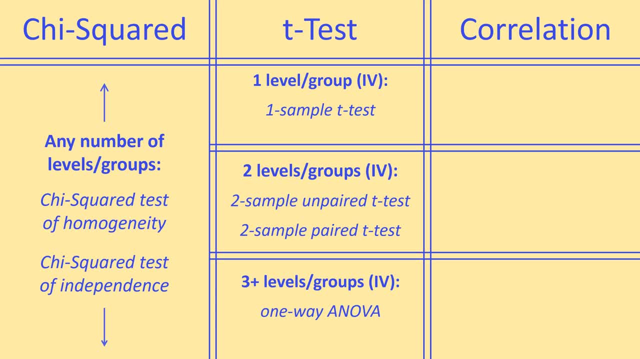 This test only looks for whether or not they're all similar or at least one is different. On to the final family. We will consider just the scenario where you have one independent variable and one dependent variable. In those circumstances, there are two primary tests you might look for. 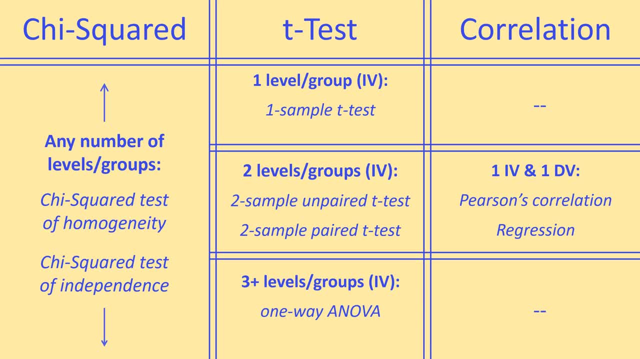 Pearson's correlation and regression Correlation tries to figure out how closely connected the two variables are. Is height a predictor of flexibility? Does age correlate with muscle mass? So it tries to understand how well those variables go together. If you know one, can you predict the other one really really well? 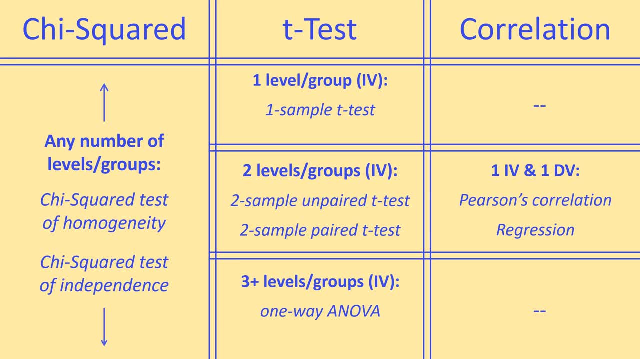 Do they correlate strongly or do they correlate poorly? That's what correlation tries to understand. On the other hand, regression tries to figure out a specific mathematical equation that describes the relationship. So it doesn't just want to know: can height predict flexibility?